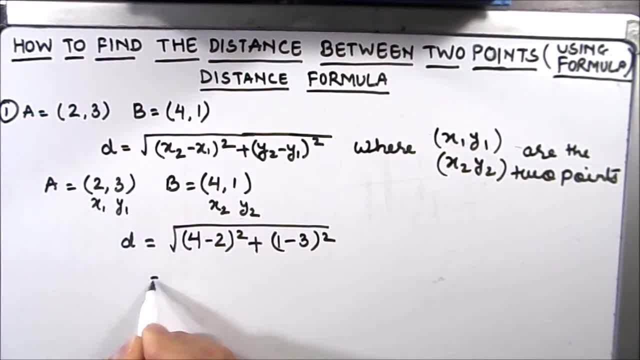 which is 3 whole square. Now we will solve this, So this will become: 4 minus 2 is 2 square, plus 1 minus 3 is minus 2 square. So 2 square is 4 and minus 2 square is also 4.. So this will come out to be 8.. 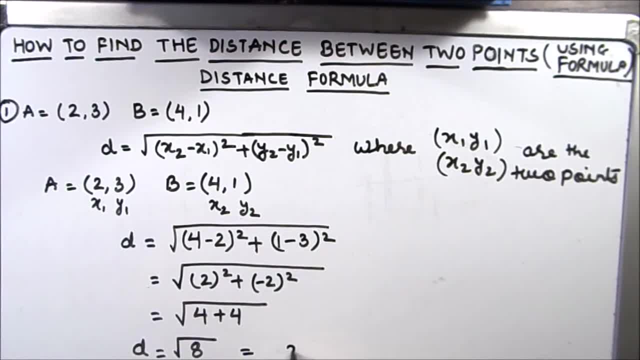 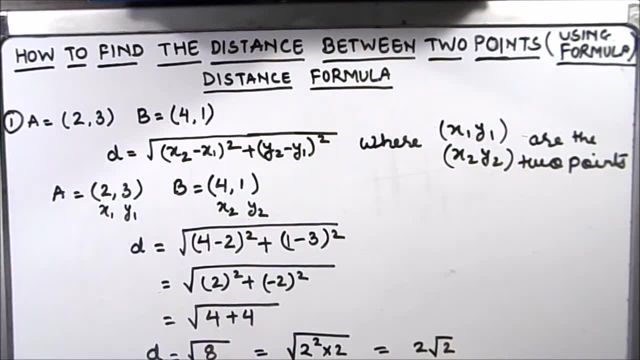 A square root of 8. we can also write as 2 square times 2 or 2 square root 2.. So our answer is: 2 square root 2 is the distance between the two points a and b. Now let's try one more example. 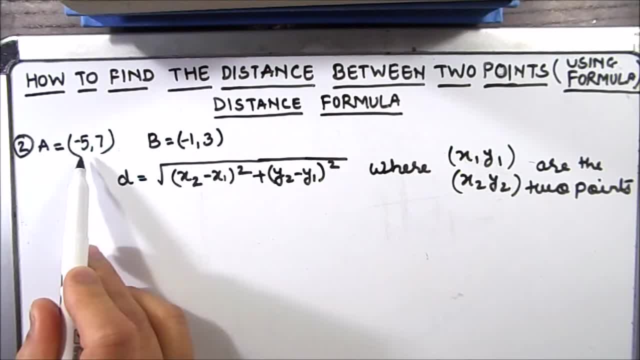 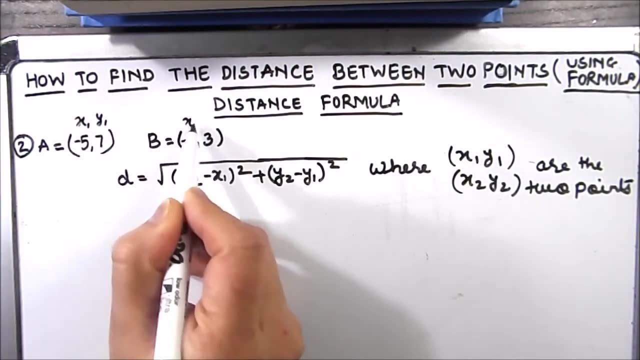 So this is our second example, where we have been given two points as minus 5- 7, and minus 1 and 3, and we need to find the distance between these two points. So first we will mark our first point as x1- y1 and second point as x2- y2.. 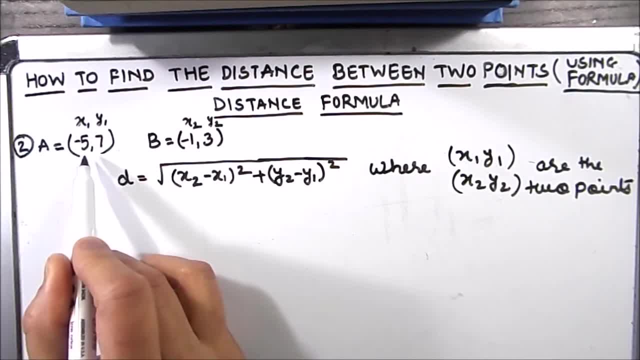 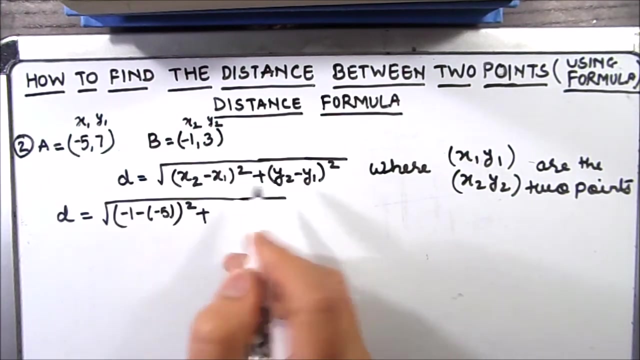 You can mark b as x1- y1 and a as x2- y2.. This will not make any difference in the answer. So let's put the value here in the formula: x2 is minus 1 minus x1, which is minus 5 whole square plus. so y2 is 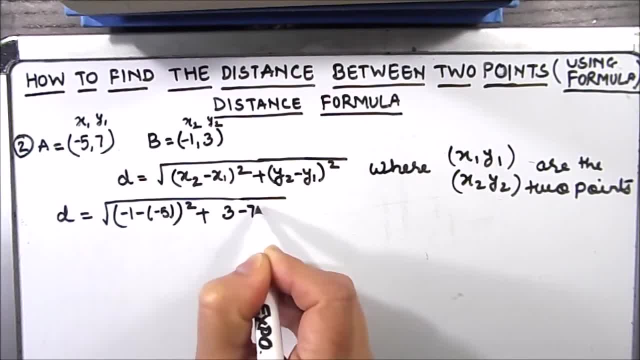 3 and y1 is minus, y1 is 7, so 3 minus 7 whole square. Now we will solve this. so this is minus 1 plus 5 whole square. plus minus 4 whole square. Minus 1 plus 5 will become 4, 4 whole. 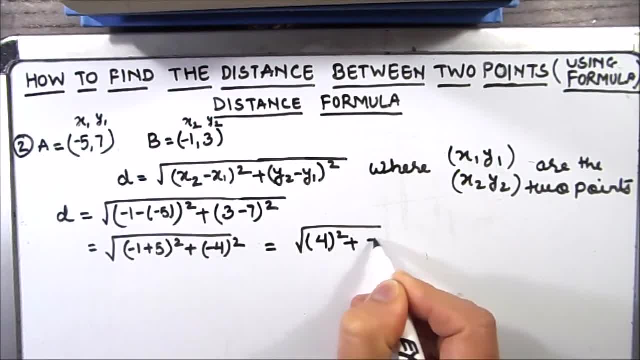 square and this is minus 4 whole square. So 4 square is 16 plus 16, which is going to be square root of 32, which can also be written as y2.. Also be written as 2 square times 2. square times 2, which is equal to 2 times 2 root 2.